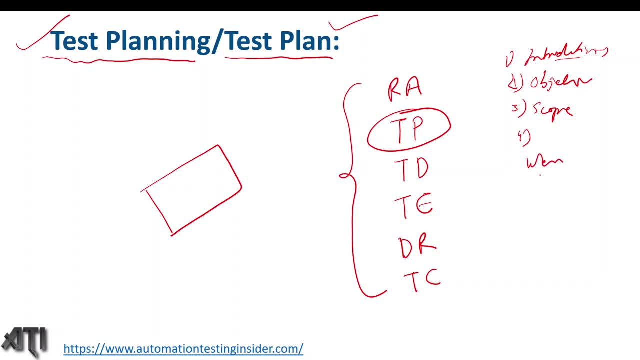 So basically, we'll discuss about when to test the application, What to test and who will test. who will test is nothing but the resources: when to test, the schedule of the testing and what to test like. what are the items are there for testing, like any school and out of school. So these are the different sections of test plan, guys, which we'll discuss in coming slides one by one. 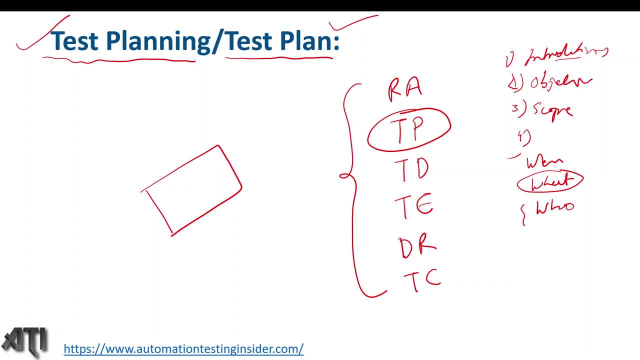 There are around 15 sections are there in test plan. It will be more or less as well, depends on the project or company, company to company as well as well. so let's talk about uh. first thing like: what do you mean by test planning or test plan? 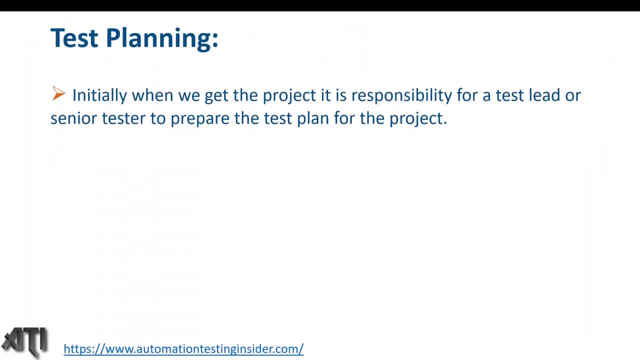 so let's get it started. so initially, when we get the project, it is responsibility for a test lead or senior test to prepare the test plan for the project. so who will prepare the test plan? so it is the responsibility of test lead and senior test engineer, senior test tester, to prepare the 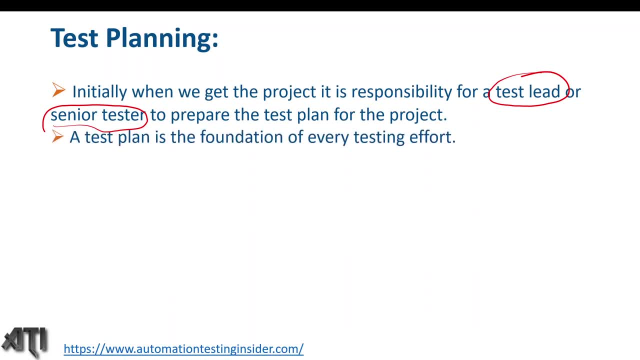 test plan for the project. a test plan is foundation of every testing effort, so this is most important, important step of any testing activities or any testing life cycle. like test planning, so test plan is the foundation of every testing effort. a test plan refers to a detailed document that catalogs the test strategy, objectives, schedule, estimations. 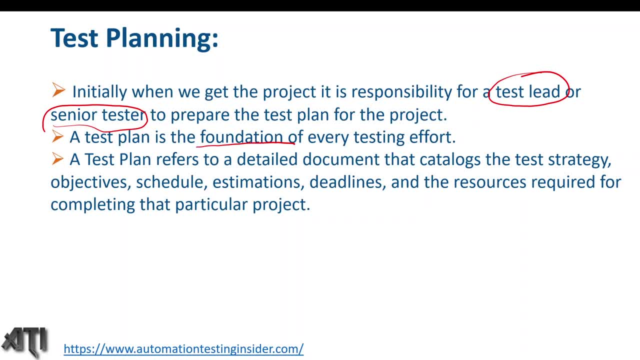 deadline and the resources required for the completing the particular project. so it talks about test strategy, right? so in in bigger projects we have test strategy document as well, which is at company level, and test plan talks about the uh project level. so this will basically talks about strategy document. basically talks about how to perform the 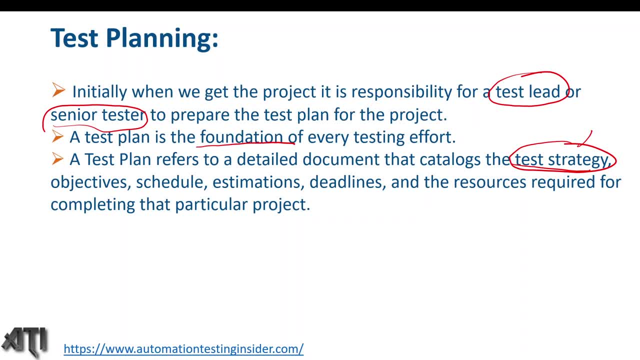 testing like. what are the techniques uh should be to be used for testing activities, to perform the testing right and in a small project. this is the section of test plan itself, so test strategy is the part of test plan in smaller, in small projects. so basically, i'll create a separate video on test strategy as well and i'll talk about the 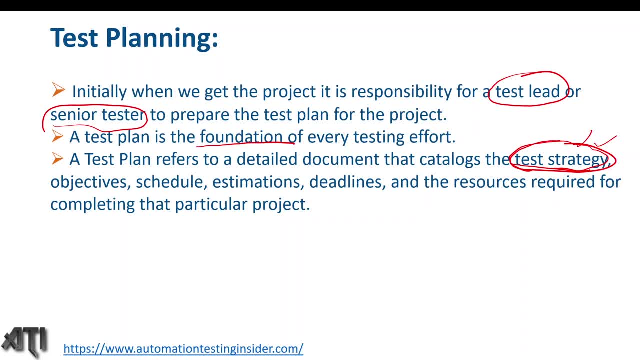 difference between test plan and test strategy. moving forward, uh, let's talk about one more thing. like a good test plan clearly defines the testing scope and its boundaries. you can use requirements specification document to identify what is included in the test plan and test strategy or the test plan statement. you can use the test plan template information to identify what is. 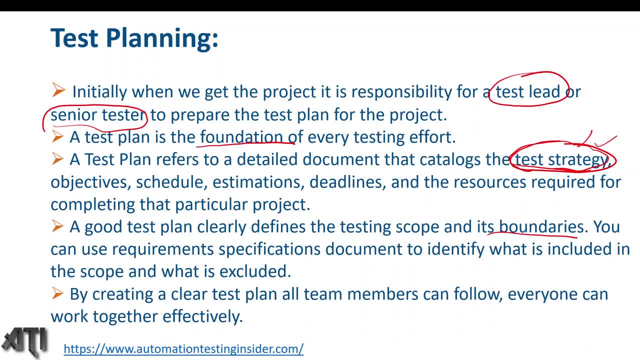 included in the test plan scope and what is excluded. so in test plan, scope should be defined clearly, like what are the items should be in scope and what are the features which is not in scope. by creating a clear test plan, all the team members can follow right and everyone can work together. 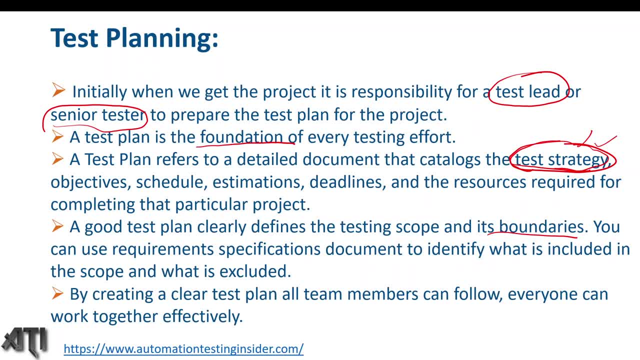 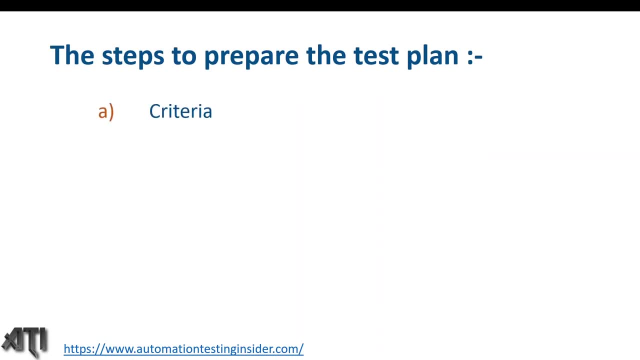 effectively of test plan is to, I mean, just configure all the activities in test planning right, so all the process should be in proper place. the steps to prepare the test plan. so what are the different steps to prepare the test plan? so the first thing is criteria, or you can say prerequisite criteria, to prepare the 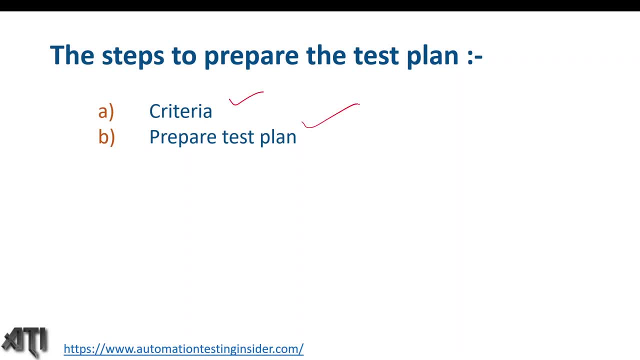 test plan. so cry. first thing is criteria, and then second is prepare the test plan, and third is get the approval of the test plan from the test manager. once it is done by senior test member or test lead, then it should be approved by the manager or test manager. so what are the criteria, guys, to prepare the test plan? 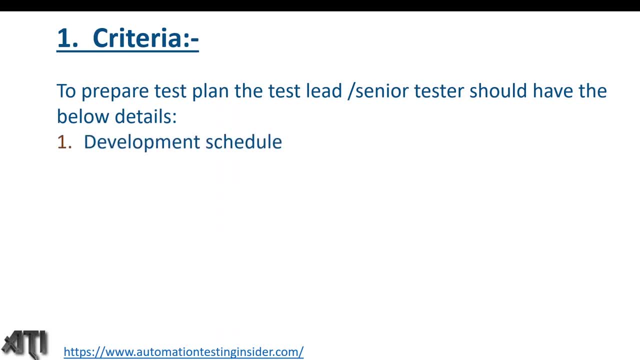 the test- lead or senior test- should have the below details: so development schedule. so we should clearly understand, like when the development starts, for when the developer are starting developers starting the coding of the particular project or a particular application. so we should come clearly know, I mean we should understand- the development activities and the schedule. 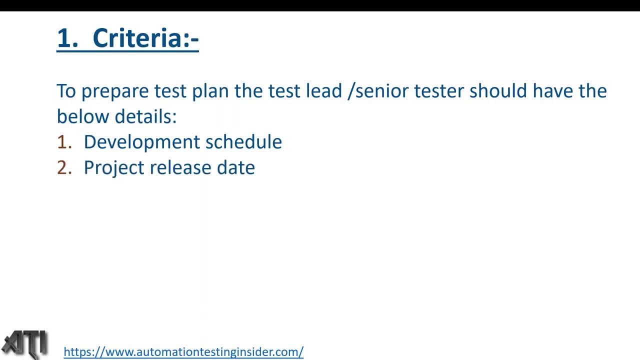 of the development so that then we can go for the test plan project release date. we should know the deadline of the project service to be, services to be provided to the customer. what are the services we are going to provide to the customer? understand the project requirements. that is very, very much. 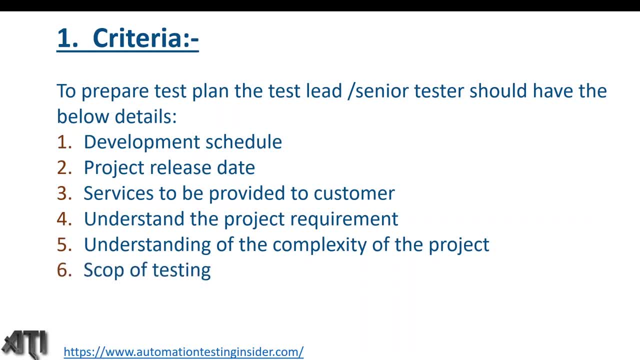 important understanding of the complexity of the project. scope of testing: what are the features which are which should be included and which are not to be included? that is scope and out of scope, number of resources required. so these are the different things, guys. another thing is type of testing to be. 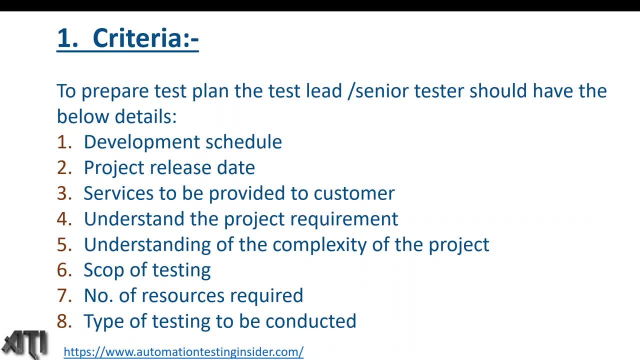 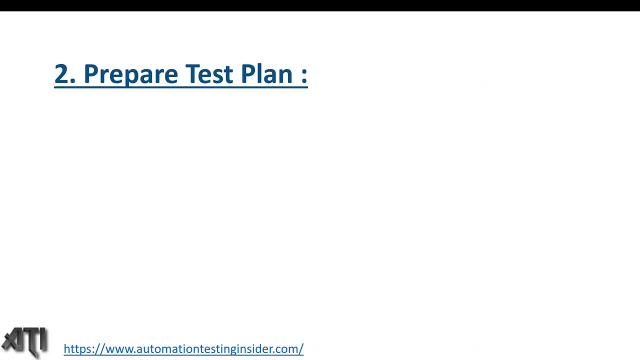 conducted, what kind of testing which we are going to perform for particular project. then the second thing is pre-requisite criteria to prepare the test plan. so until unless, if we don't know this criteria, then it's very difficult to prepare the test plan. the second thing is prepare the test plan how we are going. 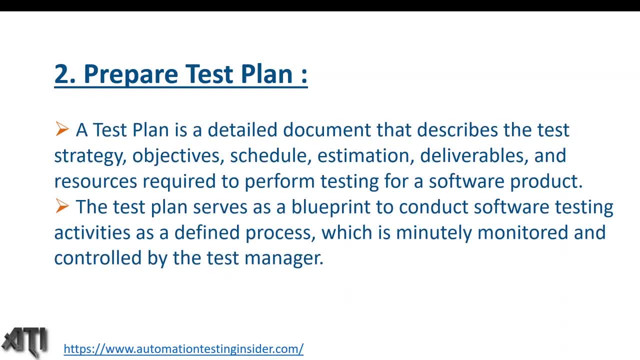 to prepare the test plan. so a test plan- this is what we have discussed. the test plans- serves a blueprint to conduct soft- test testing activities as defined process which is minutely monitored and controlled by the test manager. so once we define every activities in test plan, we can use them so in our test. 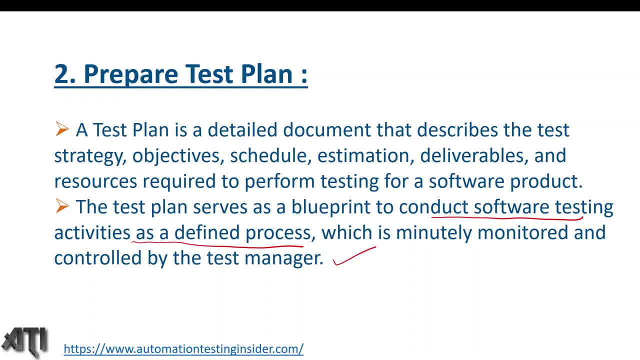 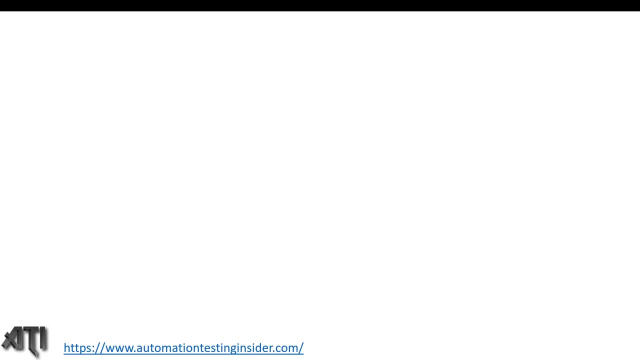 so that will be monitored by the test manager whether every activity is in place or not. so that is the purpose of the test plan. so this is how we prepare the test plan in the second part, and third is get the approval once. so there that there are three things. first one is prerequisite. 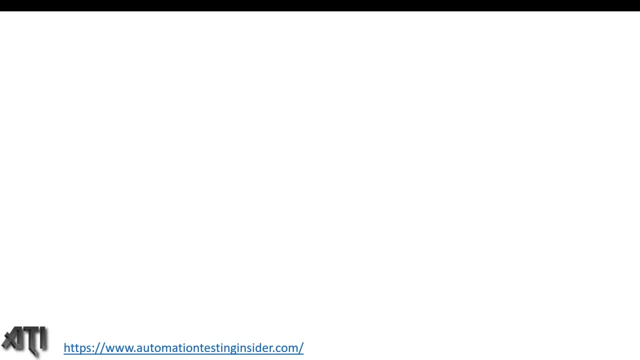 criteria. second is: prepare the test plan and get the approval. the third point: now let's talk about what are the different sections in a test plan? so test plan document has to: uh, has the has the below details right. so we have introduction features to be tested. that is nothing but. 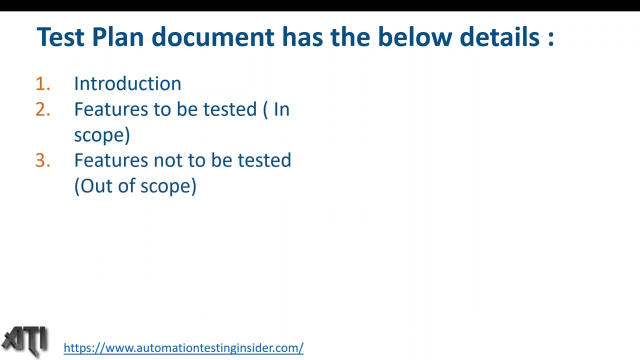 in in scope? what are the features? are in scope feature not to be tested out of scope? pass fail criteria and entry exit criteria. we, what is the approach of testing? what is schedule of testing? what are the test factors? resources who are, uh, what are the resources which we are working for? 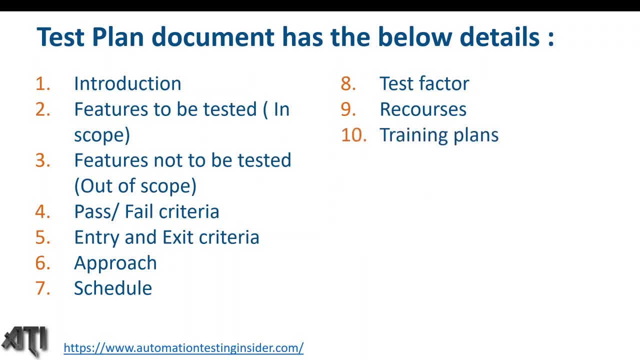 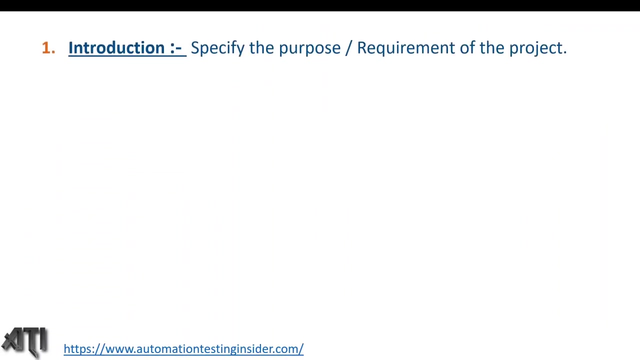 that particular application or project training plans, configuration management, test deliverables, test environment, risk and mitigation plan. and last one is approval of the test plan. so these are the different things as part of test plan, guys, so let's talk about them one by one in detail. so introduction. so specify the purpose, requirement of the project. 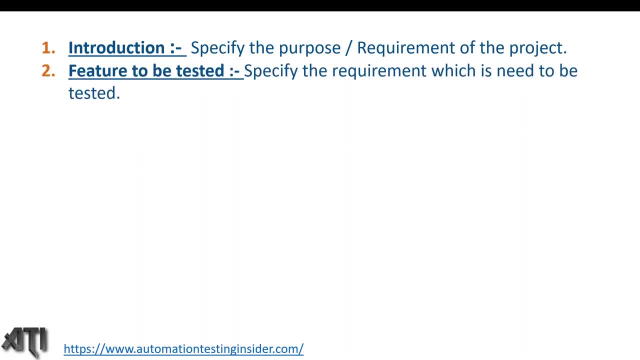 is nothing but the introduction. like there will discuss, uh, talk about what is the, what is the client name, what are the requirement of the project. so that is part of introduction: features to be tested. specify the requirements which need to be tested. uh, which are in scope features, not. 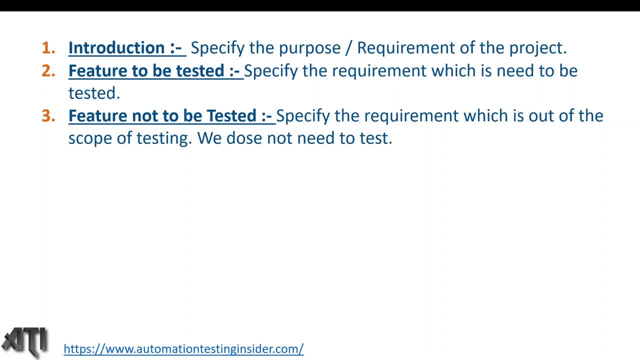 to be tested. specify the requirement which is out of the scope for testing. we do not need to test. there is a spelling mistake over here. we do not need to test pass fail criteria. so i'll provide the notes in the in my blog: guys: automation testing insidercom. 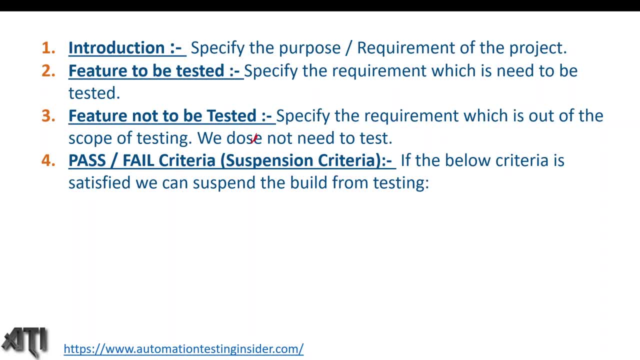 do not worry about that. all these nodes. so pass fail criteria. so what is the pass fail criteria? so there is a section called pass fail criteria, or you can say suspension criteria, in test plan. so if the below criteria is satisfied, then we can suspend the build from testing. if the build is not, 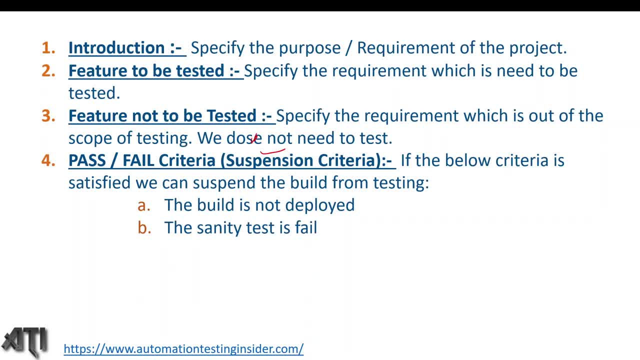 deployed, so we cannot test the application. the sanity test is failed, so we cannot go for. we cannot go for the further testing if the build is unstable. this is another criteria which we cannot go for: the further testing. wrong build is given- and there is a note here- if the build is suspended. 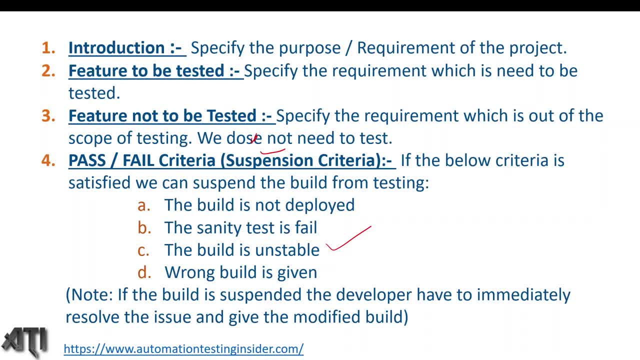 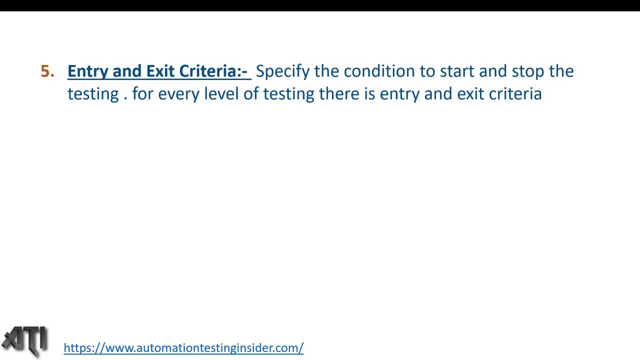 the developer have to immediately resolve the issue and give the modified build. so these are the pass fail criteria. so until unless if this criteria is satisfied, then we cannot go for the further testing. so this is another section in test plan document guys: pass fail criteria or suspension criteria, entry and exit criteria. so specify the condition to start and stop the. 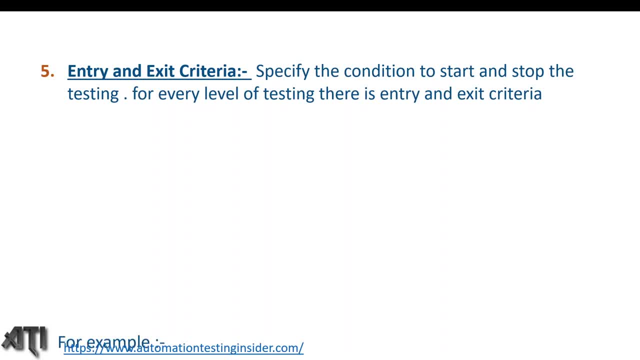 testing. for every level of testing there is an entry and exit criteria, for example. so we have different levels of testing. we have unit level of testing, integration, system level and acceptance level. now here i have given any example of system level system testing, entry criteria. so integration testing should be completed. all the major defect found in the integration testing test. 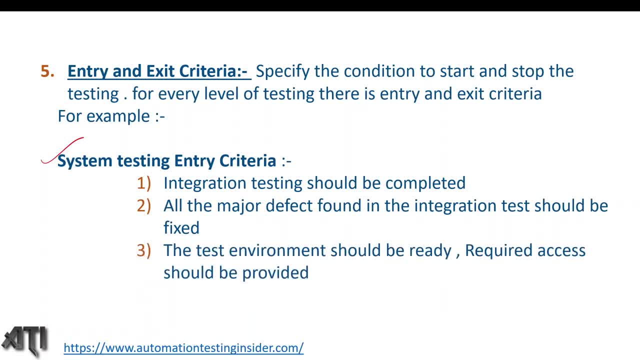 should be fixed, the test environment should be ready, required, etc. for so many community. keep on test, be happy and I will see you soon. bye, bye should be provided. the development should be completed. all coding should be done at this point of time, so whenever we get the build for system testing. so 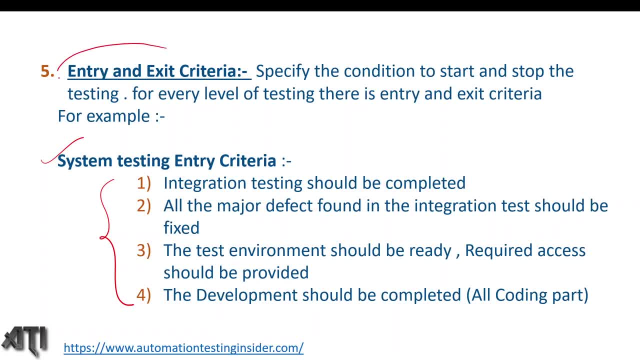 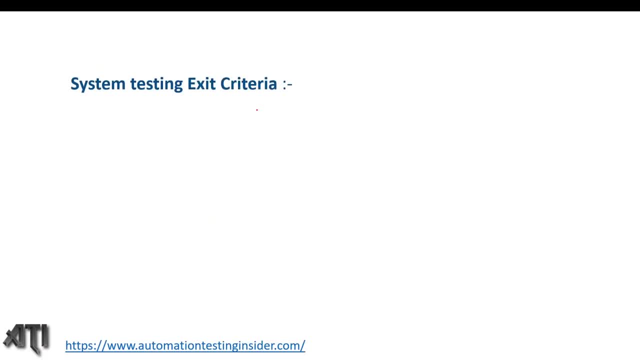 all these criteria should be satisfied. so this is another section in test plan: entry and exit criteria. now let's talk about this is entry criteria. now let's talk about exit criteria. all the functionalities are tested. no new defects are found, no risk in the project. all the defects are fixed. the testing: 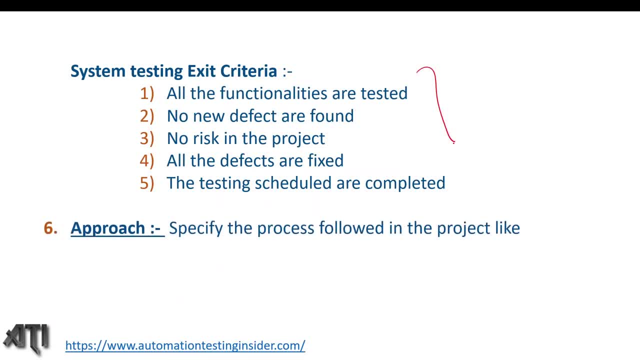 should schedule are completed. so these are the exit criteria. so once this, these are satisfied, then we can go for the further, for the testing right, once all these criteria are satisfied. so this is exit criteria in system testing. now approach: specify the process followed in the project, like: what is the approach. 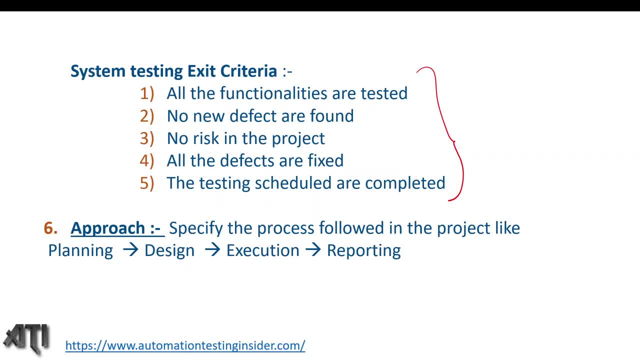 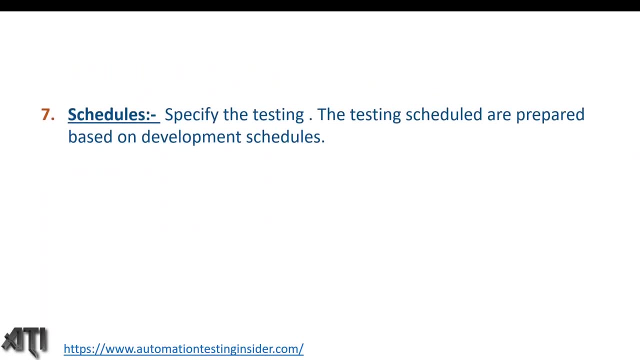 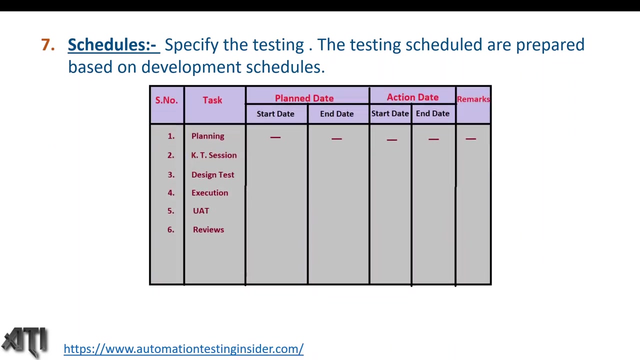 which we are going to follow for particular project as part of testing activities, like what is the plan, design, execution and reporting. so this is the approach of testing should be defined in the test plan schedule. specify the testing. the testing scheduled are prepared based on development schedule. right, so it should. 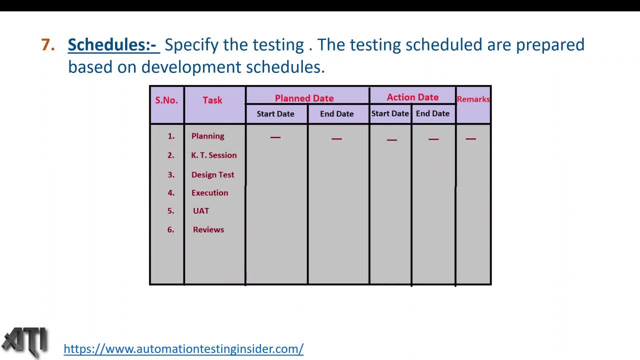 be based on the development schedule, because testing is the part of development activities. we have requirement analysis, design, coding, testing, release and maintenance. so ultimately, testing is the part of development schedule. so when we talk about schedule, so if you talk about the test plan schedule, so we have planning KT session. 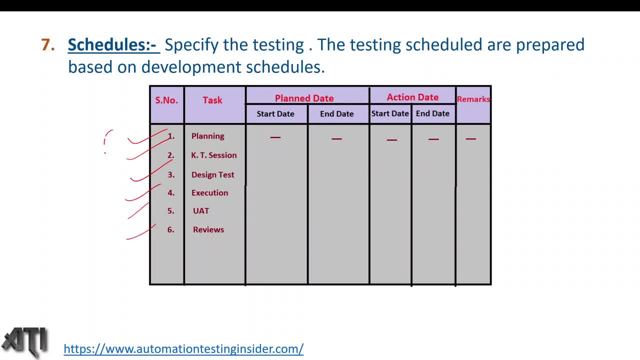 design, test execution, uat reviews. so these are the different task, correct? all the testing lifecycle should be listed down here, like: what are the activities which we are going to perform, what are the tasks which we are going to perform, like planning of the testing, the KT session, KT session testing, test planning. 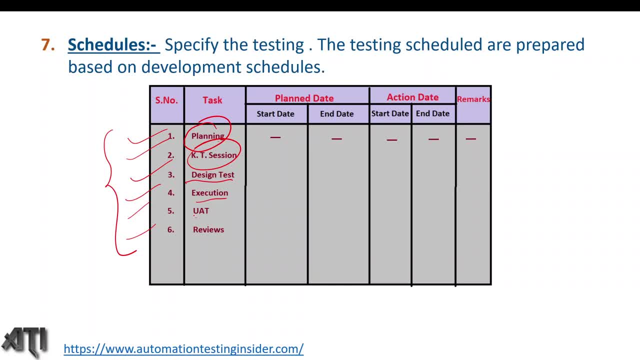 to the resources, design, the test, execution, uat reviews. so these are the plan dates. what is the plan date? what is the end date and what is the actual actually started and ended action date? you can say action date or actual date and if you have remarks, we should put some remarks over here. 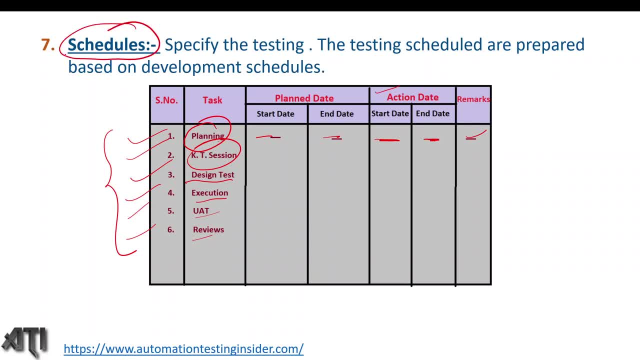 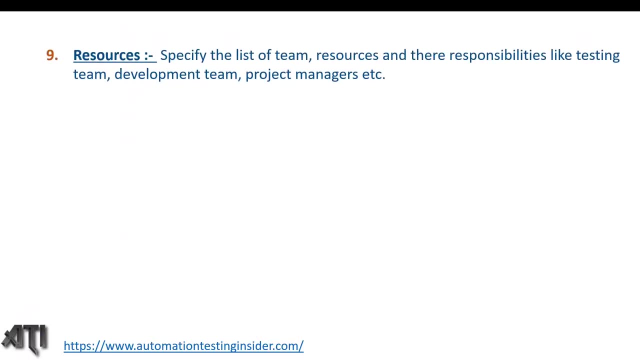 as well. so this is important part of test plan schedule. now let's talk about another one: test factors. so identify the test factors required for the project resources. this is an important part of test plan resources. specify the list list of team resources and their their responsibilities like testing team. 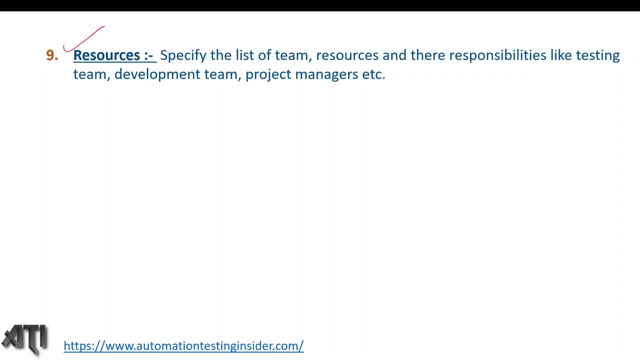 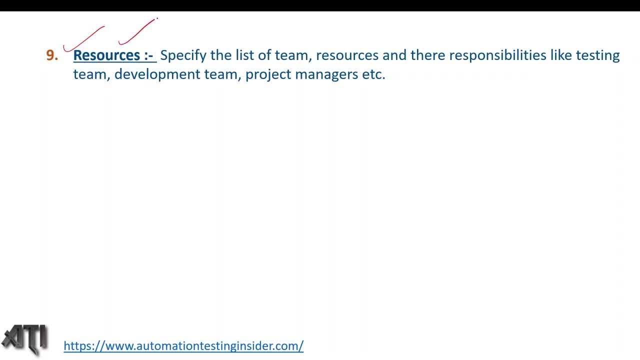 defined in the test plan. so this is another section, guys, important section of test plan, training plans. so specify: any training plan is required for the resources. okay, what are the trainings, what are the further skills required for the resources? so that should be carried out as part of training plan: training, training plans section in the test plan: configuration management. 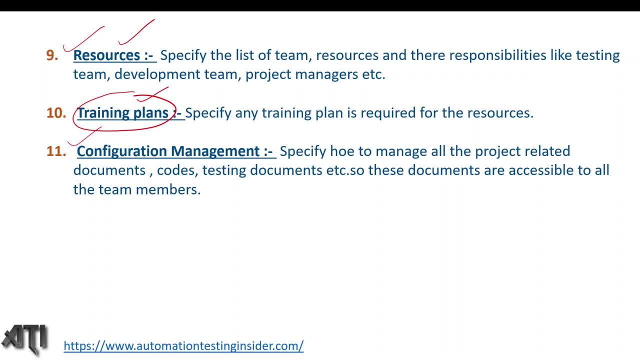 so So specify to manage all the project related documents- coding codes, testing documents, etc. So these documents are accessible to all the team members. So there should be a repository where we can access all the documents or codes. In case of automation testing, we should get the codes from GitHub. 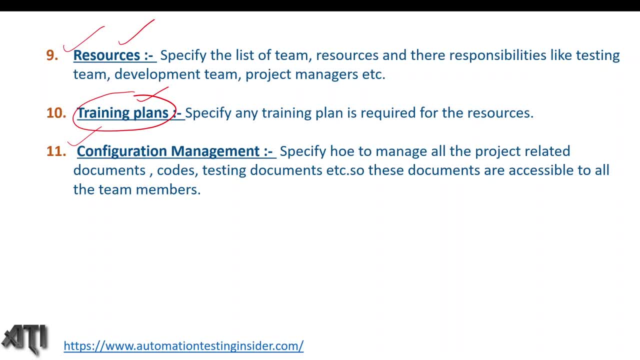 GitHub is another. I mean one kind of repository where we keep all the documents We have SharePoint. Nowadays we are using SharePoint And to keep the codes we have GitHub. So these are some configuration management tools, guys, And there are long back we used to have VSS, Visual Source Save. 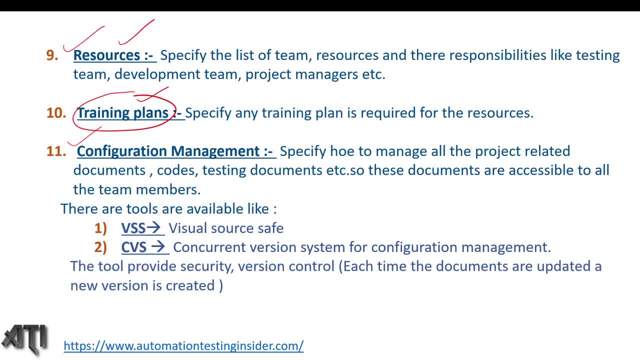 We have concurrent version system, So the tool provides security, version control. So what do you mean by version control? So each time the documents are updated, a new version is created. So, if you remember, we have version control. 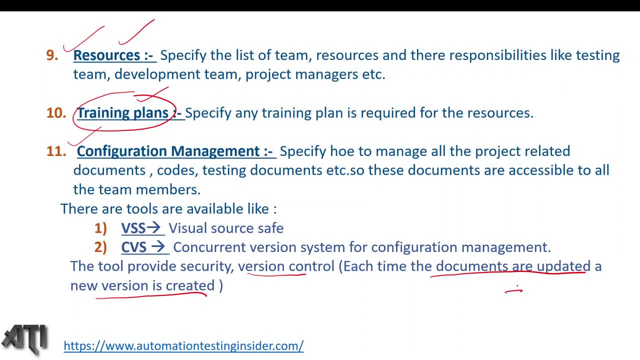 Whenever we update the system, Update our documents, So there should be version created. Let's say, this is version 1.. There should be version 1.1, 1.2, 1.3, like this, So we can access any of the version anytime. 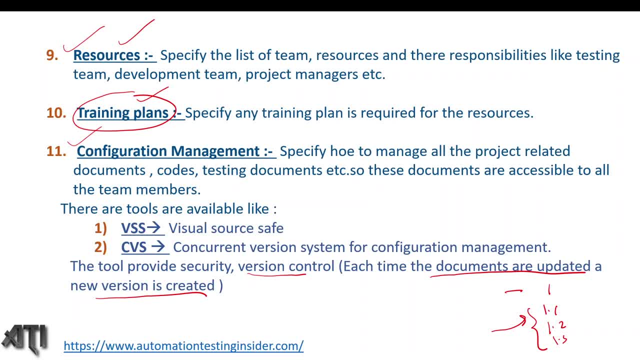 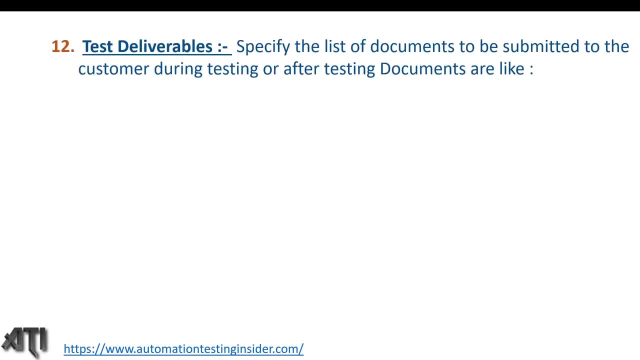 That is the main important point of configuration management: Test deliverables. So this is another important section of test plan guys. So specify the list of documents to be submitted to the customer during testing phase Or after. the testing Documents are like test plan, test case documents, test cases, test execution results, defect report, review report, test summary reports, etc. 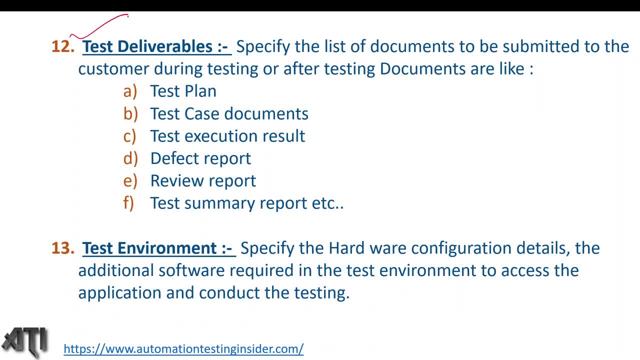 And yeah, So this is another section of test plan. We have one more test environment. Specify the hardware and software configuration details over here. Hardware configuration details: The additional software required in the test environment to access the application And conduct the test. 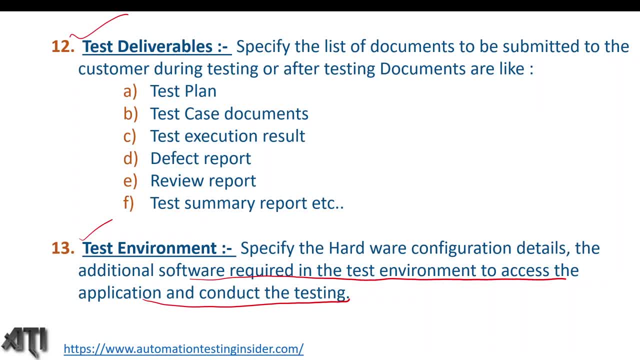 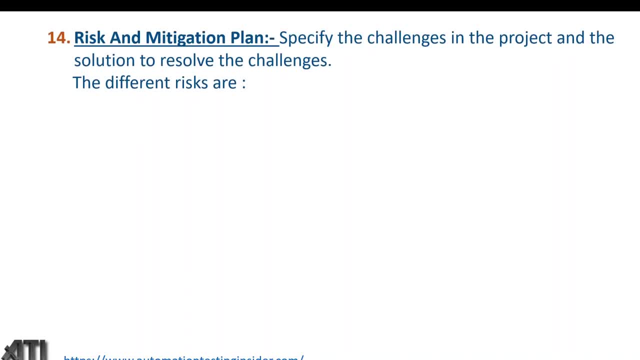 Testing. So testing environment should be specified, And this is another section of test plan. What are the risk and mitigation plans? So specify the challenges in the project and the solution to resolve the challenges. So the different risks are required. documents are not available. 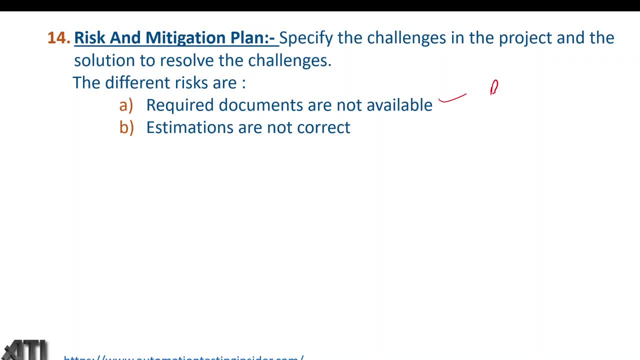 Estimations are not correct. Let's say, if we don't have requirement like BRD documents, So that is risk. We don't have requirement document from the customer right Or from the BA team, So we cannot author the test cases properly. 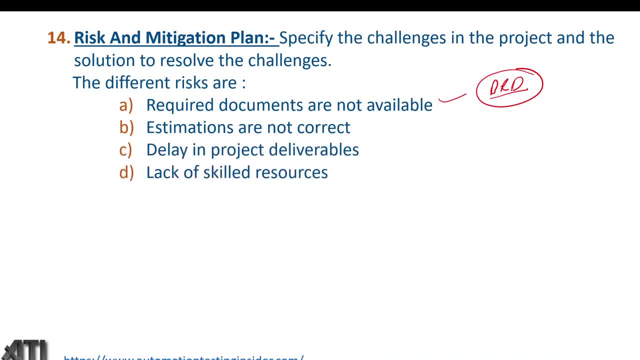 Estimations are not correct: Delay in project deliverables, Lack of skilled resources, Lack of team coordinations, etc. So these are the different risks involved in the project. So that should be carried out as part of section called risk and mitigation plan in the test plan document. 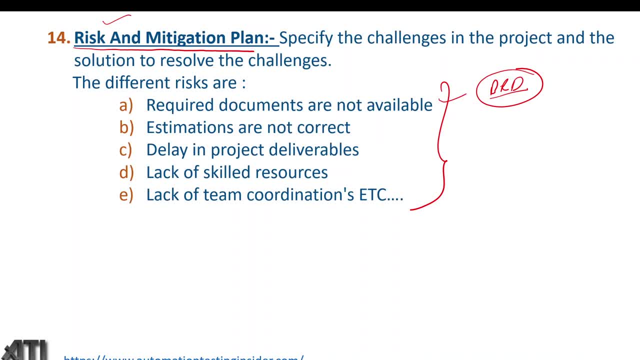 Mitigation plan is like: how to resolve those risks. What is the mitigation plan we have prepared for the different risks, What are the different risks involved in the project? and the final thing is approval- sign-off of the test plan documents. So, after preparation of the test plan, the project manager and customer have the review and approve the test plan. 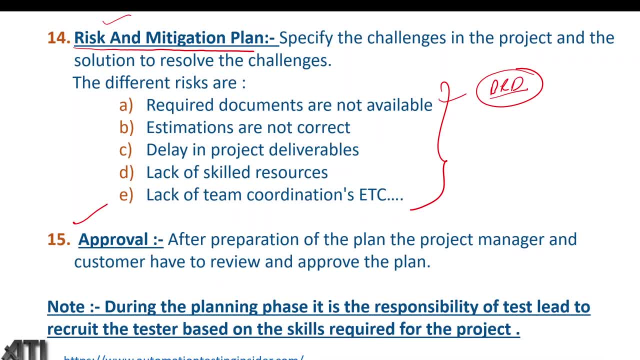 And there is a note, guys: So during the planning phase, it is responsibility of a test lead to recruit the tester based on their skills required for the project. So this is very important. So whenever we start the project, so we should have the proper, we should have them.